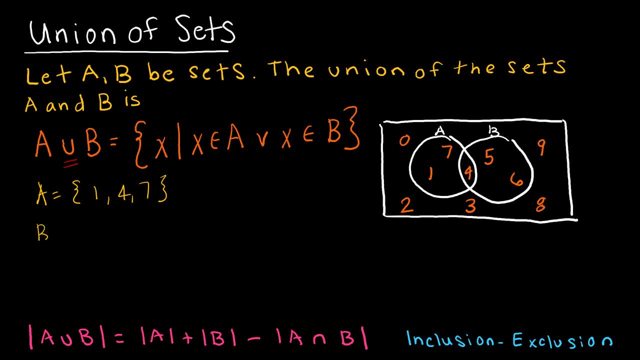 seven And set B, because that was everything contained in the set A circle: 1,, 4,, 7.. And in set B it contains the elements 4,, 5, and 6.. And so A union B would be 1,, 4,- and- notice 4 is listed twice, but I'm only going to list it once- 5,, 6, and 7.. 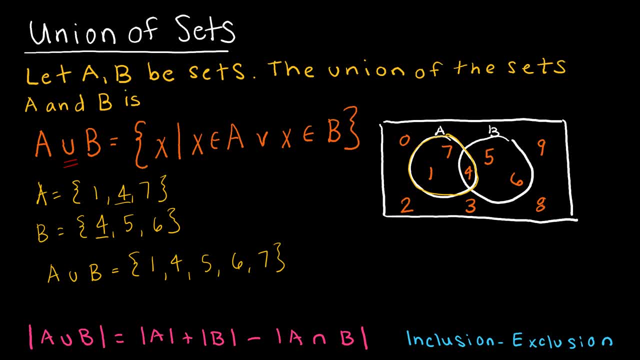 So, using my picture, it's essentially everything here in either circle, including this part in the middle that's contained in both. So 1, 4, 5, 6, 7 would be all of the elements in the union. 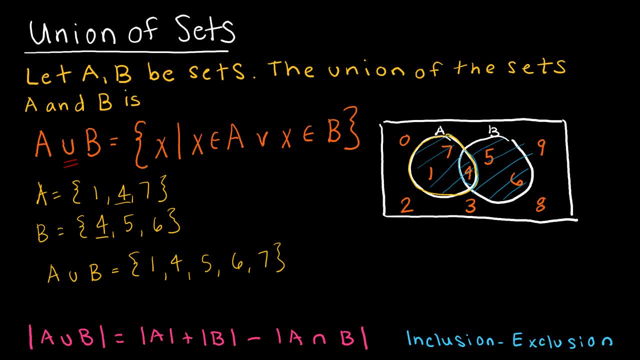 So we're looking for anything that is in one or the other. So again, you can think of this as an or Down here. I've included a set of elements. I've included our inclusion-exclusion formula. We talk a lot about that later on. 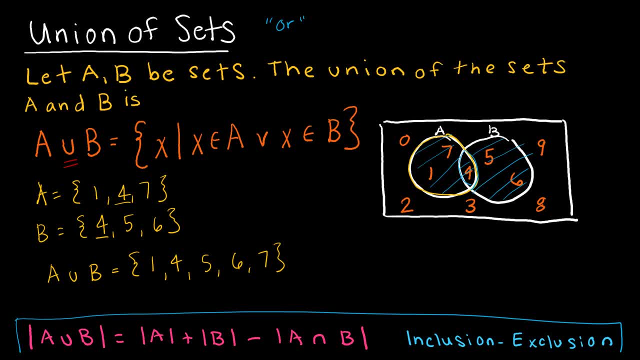 But this is essentially the formula that you would use Here. if I had A union B, I could take all of the elements of A, which would be 1,, 4,, 7. And add all of the elements of B, which is 4,, 5,, 6.. 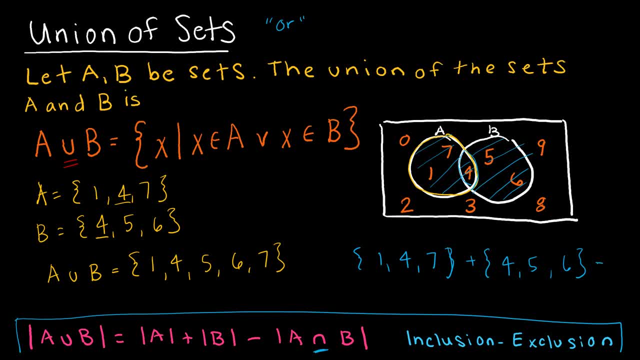 And then I'm just going to subtract. I'm going to subtract anything that's here and we haven't talked about this quite yet, but this is the intersection, And the intersection is here where it's, in both sets. so I would subtract 4.. 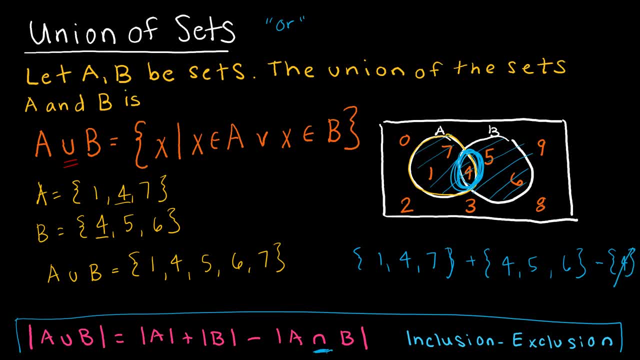 And, as you can see, what happens there is that just one of those 4s go away and I would be left with 1, 4, 7,, 5, 6,, which is the answer that I came up with before. 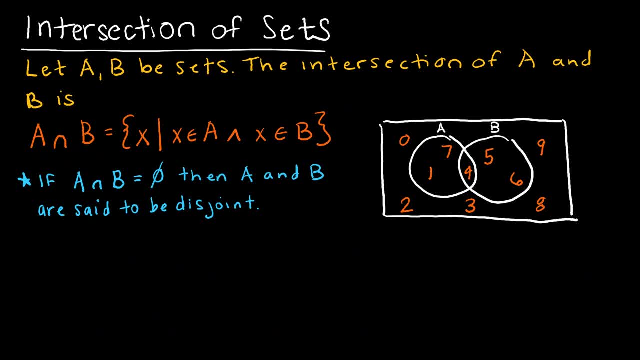 So the intersection of sets if, or, or, if the Union was sort of like an or, this is sort of like an and. And I'm saying the only way that it belongs in the intersection is if it's in set A and B. 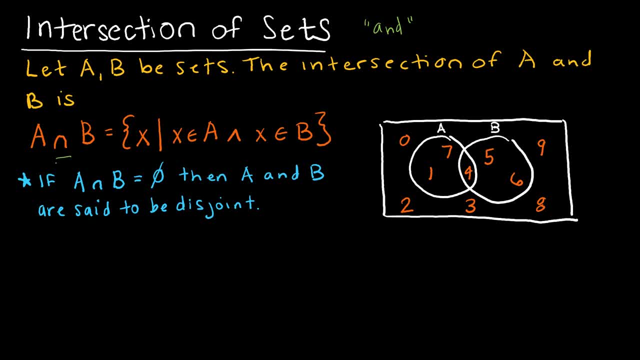 So here I'm saying A intersect, B is the set of all Xs, such that X is in A and X is in B. So looking at my picture, before we get to that part, I've written in blue. looking at my picture, I can see that the intersection 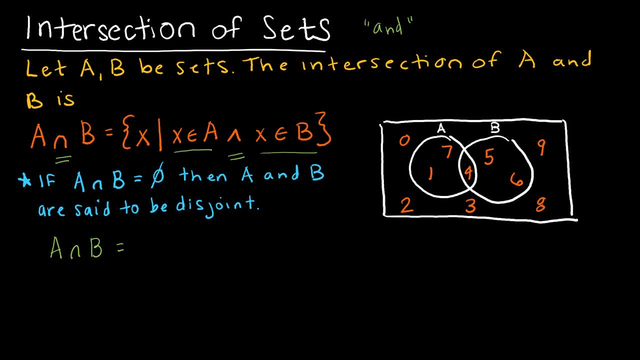 A intersect. B in this example is just 4, because here I'm looking at a 4 that is contained in A, because, remember, A was 1,, 4, 7, and B was 4,, 5,, 6, and so the intersection is only elements that they have in common, and in this case that is only the element 4.. 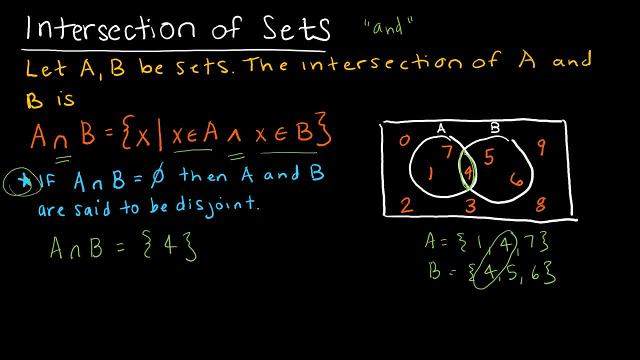 So what I'm saying over here in blue is I'm saying if the intersection is empty or the empty set, then A and B are said to be disjoint. So that's just another little vocabulary nugget that you can file away Disjoint. my Venn diagram would look more like this, because there would be no intersection or no elements that were contained in both sets A and B. 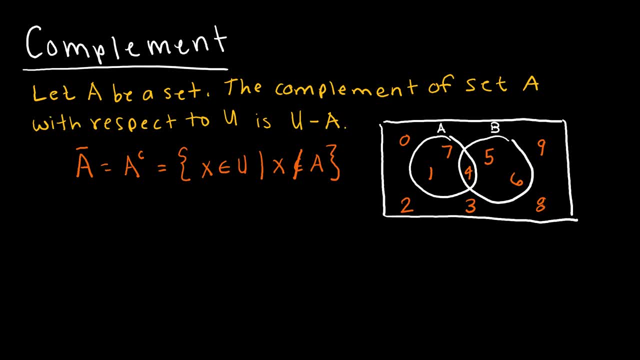 The complement is: Is another operation or another concept. that is really important to understand. and the complement of a set is essentially any elements that are in the domain or in the universe that are not in that set. So here, as you can see, I've got not A, so it's kind of like not P of X, where P of X is any element in set A. 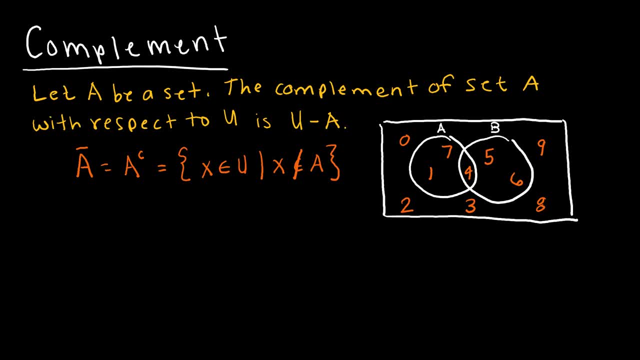 We're essentially saying: it's anything that's not A, It's anything that's not in set A, that's in the universe. So you might also see it written like this: that is the complement of A, but this is the way that I'm going to be writing it, not A. 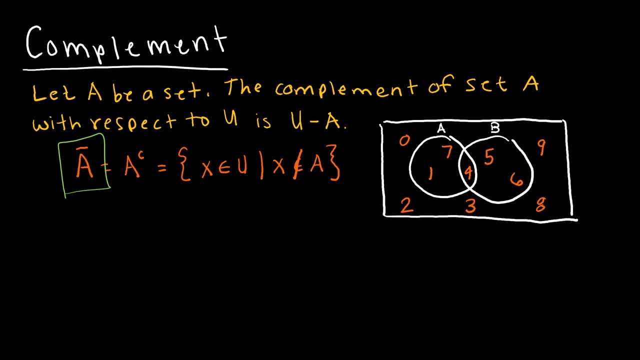 And essentially it says it's in not A if X is in the universe, but X is not in set A. So let's take a look at our picture, where I have set A and set B. So set A is everything inside of this circle, which is 1,, 4, and 7.. 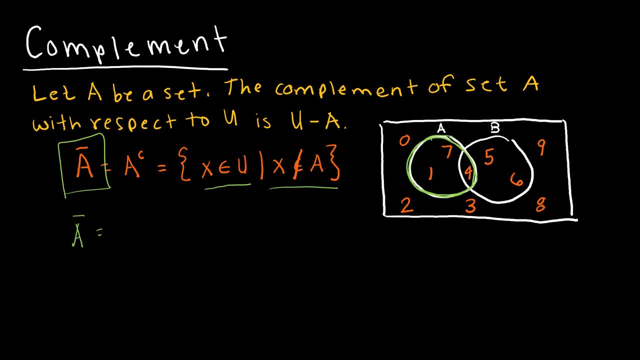 So the set not A would be any number that's not 1,, 4, and 7.. So I would say set A is 0,, 2,, 3.. Notice, these are all out in the universe. Still, 5 and 6, even though those are not just out here hanging out, they're in set B. 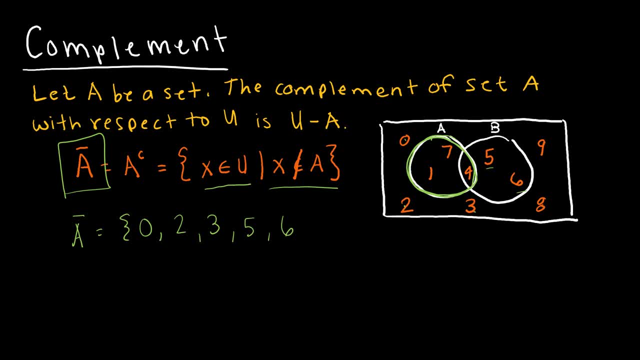 Not including the 4, but 5 and 6 are not in set A, And then of course 8 and 9.. So not A. A would be 0,, 2,, 3,, 5,, 6,, 8,, 9.. 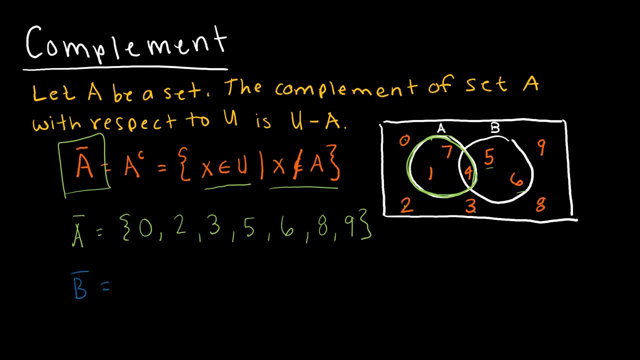 Let's say I wanted not B Again. that's all the digits from 0 to 9, but I couldn't include 4,, 5,, 6.. So it would be: 0,, 1,, 2, 3,, 4,, 5, 6 are all inside B. 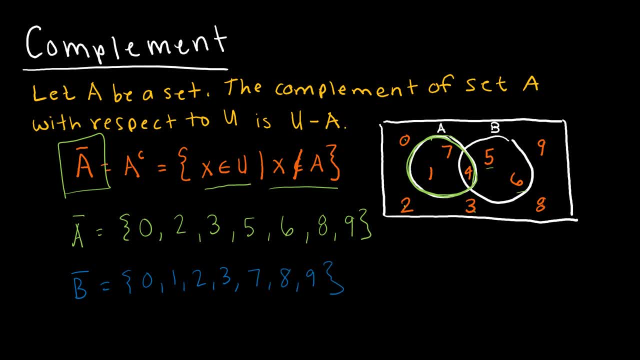 So 7,, 8,, 9.. Those are all of the not B. And of course you can get crazy and you can say: well, A union B Or not A union B. So remember: A union B. 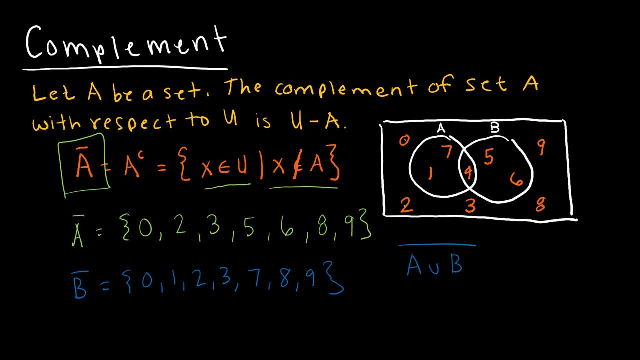 Let me erase my little markings here. A union B is everything inside A or B, So not A union B would be anything that's not inside A or B, which would be 0,, 2,, 3,, 8,, 9.. 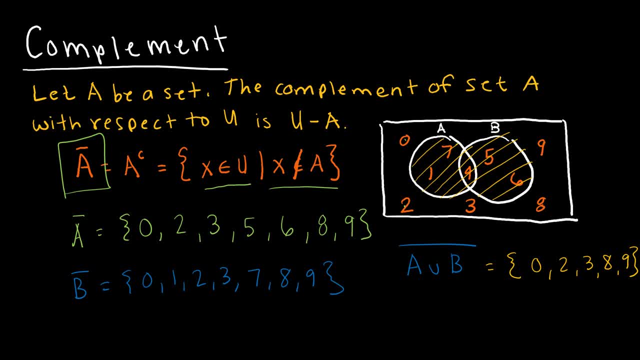 So all of those values on the outside, I could do A intersect B And not. And again, A intersect B is just this part in the middle, So not A intersect B would be everything else, which would be 0,, 1,, 2,, 3,, not 4, because that's the one in the middle. 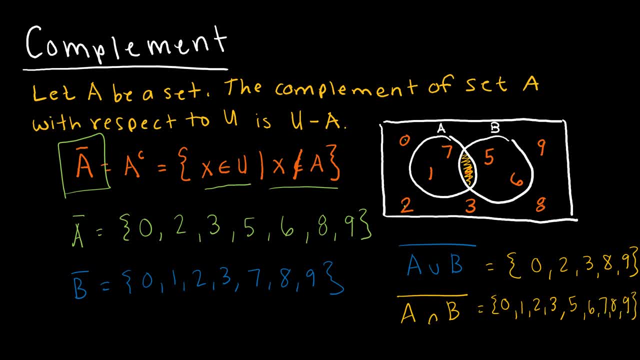 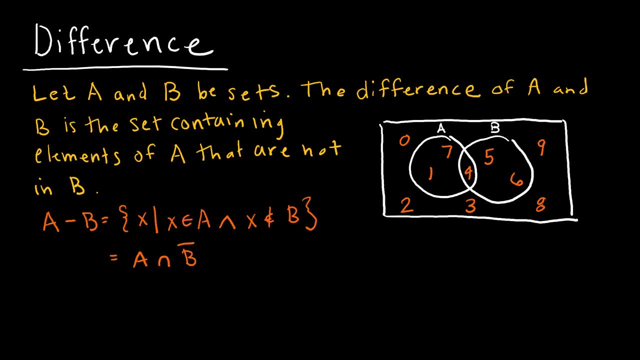 5,, 6,, 7,, 8,, 9.. So hopefully we understand the concept of a complement And we're going to now look at the difference. And the difference is essentially the set containing All of the elements of set A that are not in set B. 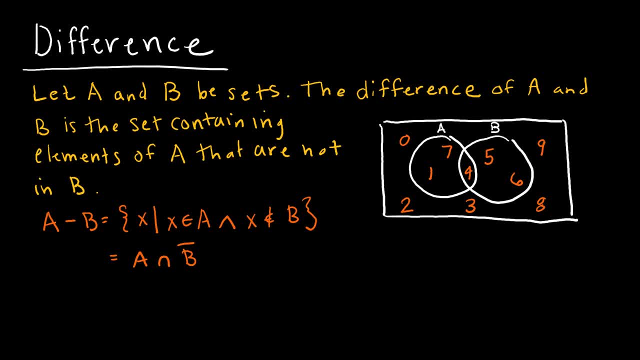 So here I'm looking at A minus B being the set of all X's, such that X is in A But X is not in B. So in this case, looking at A minus B, in my picture my only options are 1,, 4, and 7.. 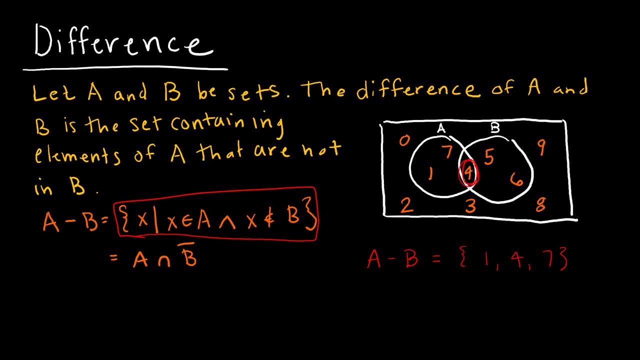 But I need to take away Any of those that are also in B, So my solution would just be 1 and 7.. So that is the or those are the values that I would use for the difference. So essentially I'm just subtracting anything that is contained in B. 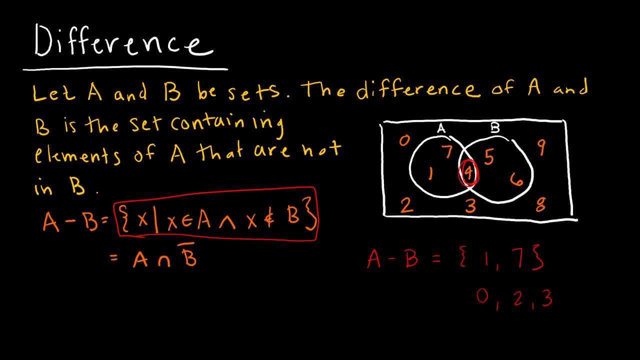 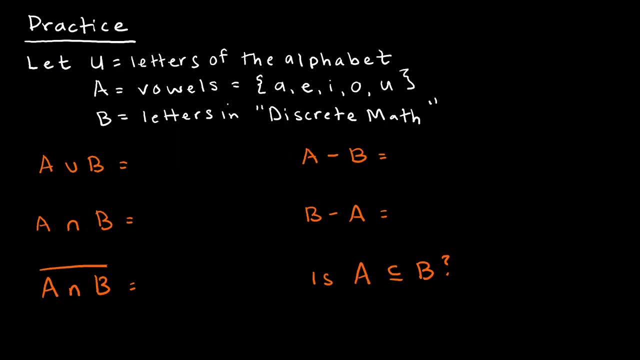 I couldn't include numbers like 0,, 2,, 3, etc. Because those were not contained in A to begin with, So it's just like a normal subtraction question. Here is a question that I would like to ask you, And I would really like for you to try. 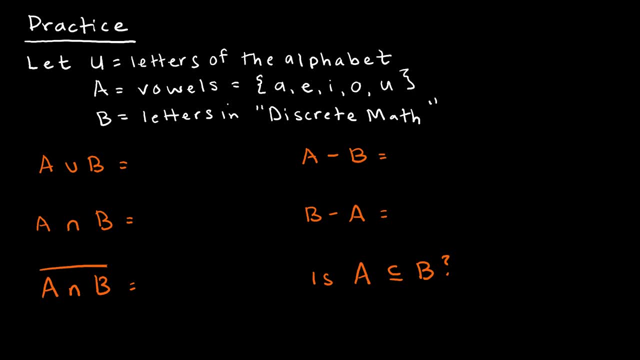 This is just a great practice question, like you might see in homework, Just to make sure you understand the concepts of, you know, subtraction or complements or unions, etc. So go ahead and press play and try this question And, I'm sorry, press pause. 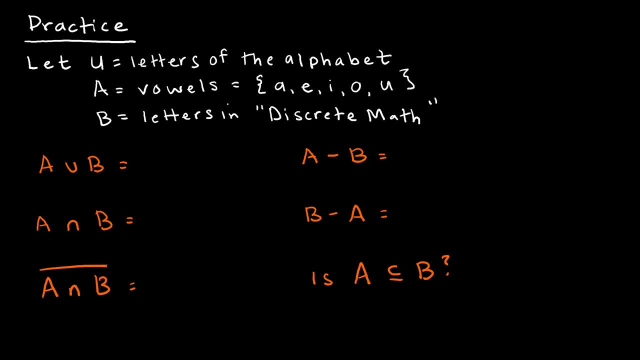 Try this question and then press play to see if your answers match up with mine. So before I get started, I really am going to rewrite Set B in roster notation, So I'm just going to list out all of the elements of that set. 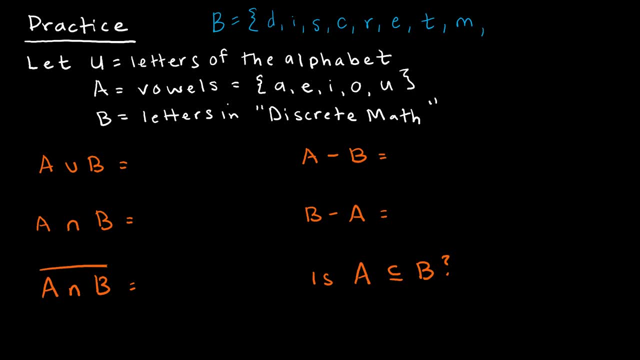 And again. I don't care for writing them more than once. So even though I've got two E's, I'm only writing E once and then M, A. I've already used T and then H And again. if I wanted to, I could certainly write those in alphabetical order. 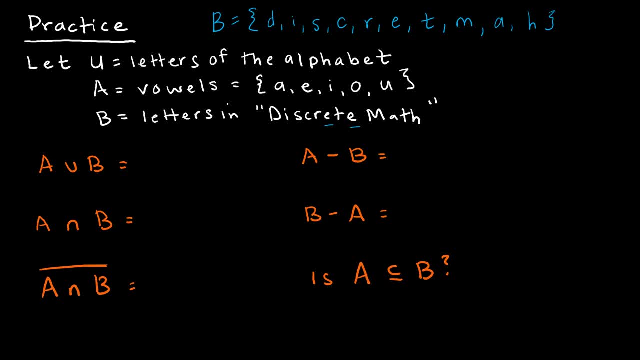 So I'm going to do that, But really it's not going to matter. So my first question asked me to find the union, And the union is kind of like the cup, And the cup contains all of the elements in either set. 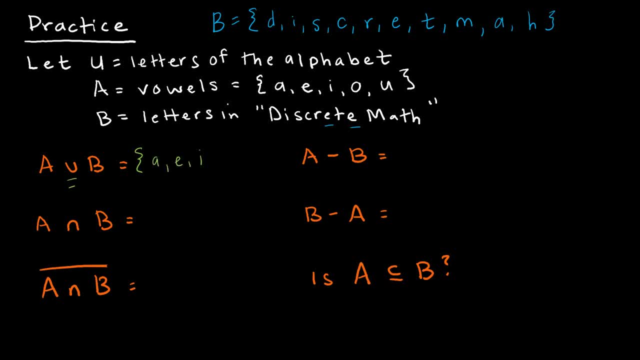 So set A is A, E, I, O, U, And then I'm going to also include everything in set B, But I don't have to rewrite A, E, I, O or U, So I've got D S, C, R. 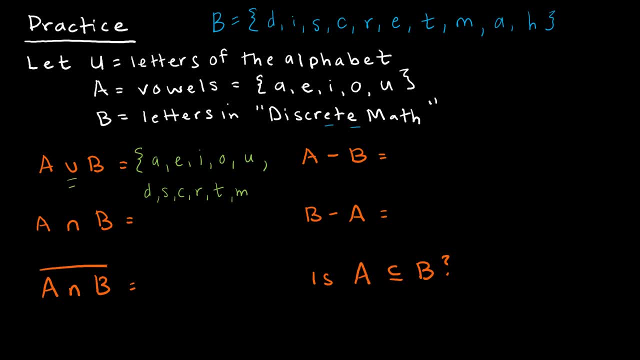 I don't have to write E, T, M, H, So all of those elements would belong to the union. The intersection would be only those elements that are in both A and in B. So I can see here I've got an A in both sets. 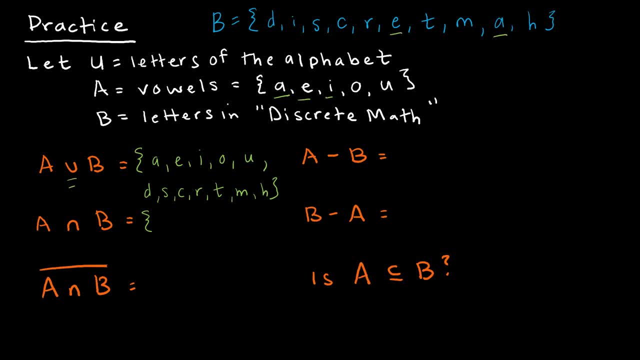 I've got an E in both sets. I've got an I in both sets. I don't have an O And I don't have a U, So the intersection would just be A E, I, And the O and U are not contained in the word discrete math. 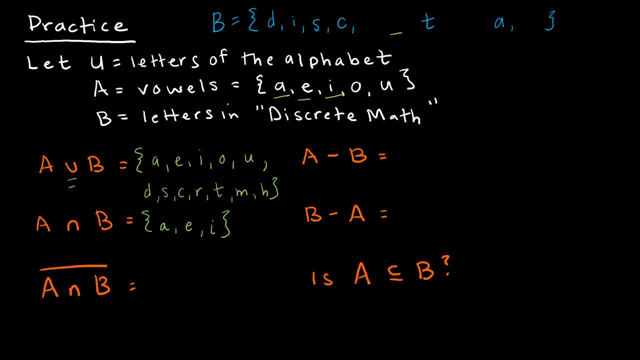 A minus B. Actually, I should have left those My bad. Unfortunately it's not going to, let me just undo. So M A, H, All right, So now I'm looking at A minus B, which is essentially starting with A, E, I, O, U. 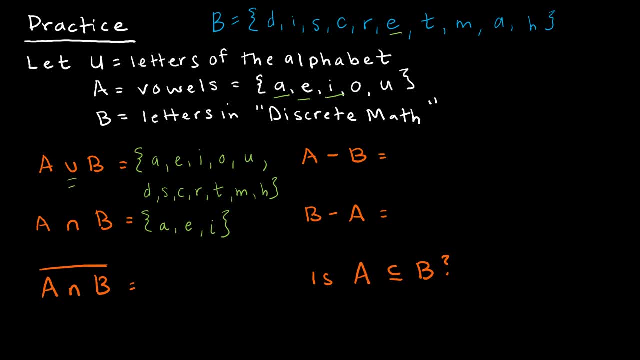 I'm saying, if I take away any values that are in B, what would I be left with? Well, it's kind of nice because I've already found the intersection And I know that B includes the values of A, E, I. 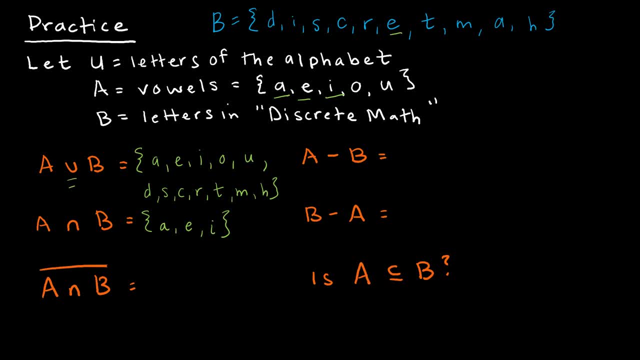 And so if I was taking A, which is A, E, I, O, U and taking away anything in set B, I would be left with O- U The other way around, starting with B but getting rid of anything that they have in common. 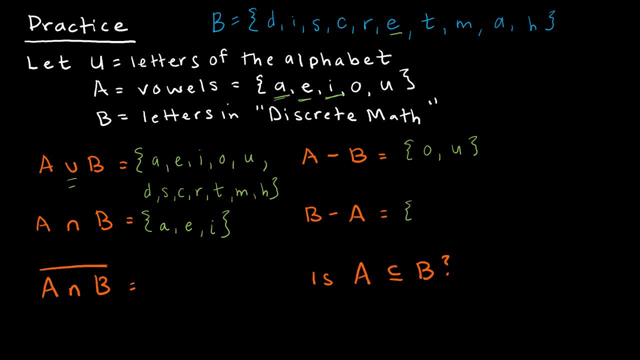 which, again, the only things they have in common are A, E, I would be the set of everything left over, which would be D. Let me just go ahead and underline that: E, I and A. So anything I didn't underline would be D, S, C, R, T, M, H. 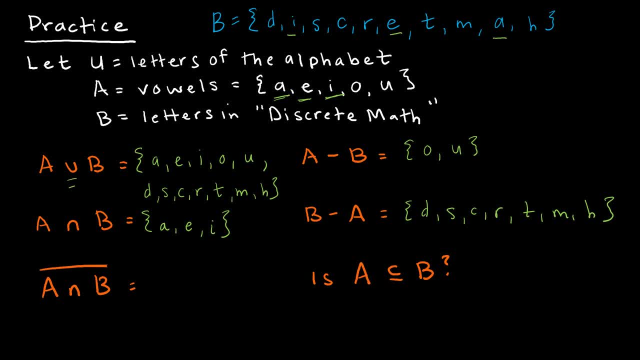 My next question says the complement of the intersection of A and B, And so, remember, the U is the universe of all of the letters of the alphabet, And I'm saying anything that's not in here, that is in the alphabet. So my solution there would be B, C, D. 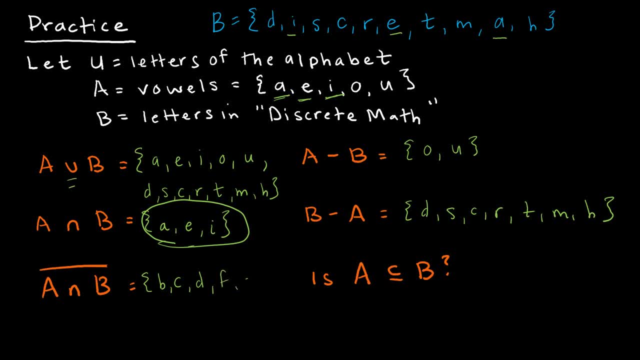 So I skipped A, I skipped E, F, G, H, I'm going to skip I, J, K, L, M, N, O, P, Q, R, S, T, U, V, W, X, Y Z.